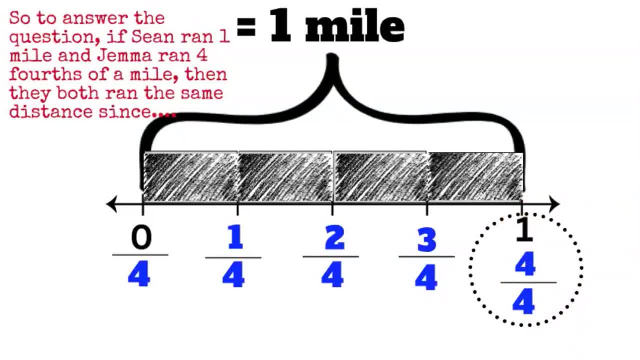 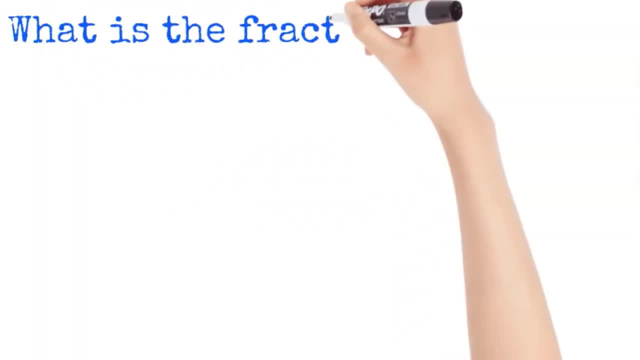 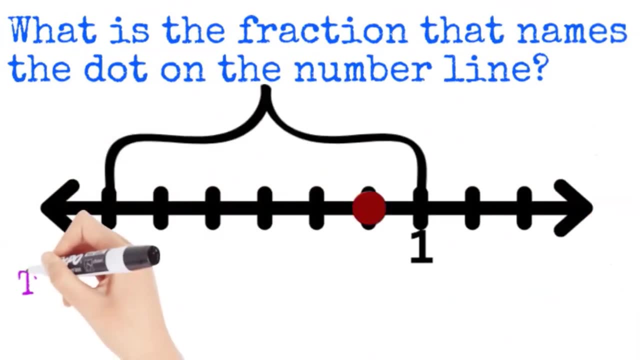 ran the same distance. since one whole is the same as four-fourths, When your numerator denominator are the same, then it's one whole. Let's try this one. What is the fraction that names the dot on the number line? Remember, the number line shows zero to one and the whole is: 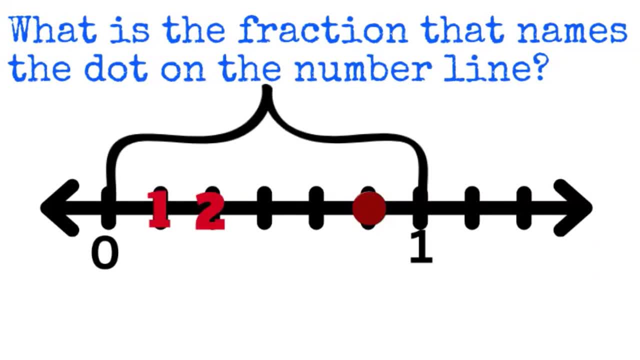 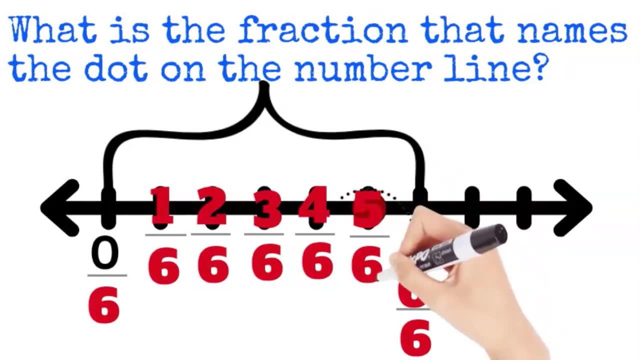 always from zero to one, So we're going to break the whole into pieces to figure out our denominator. In this case there are six equal pieces, So six is my denominator. There's one, six, two, six, three, six, four, six, five, six and six, six would be my whole. However, the dot is on five. 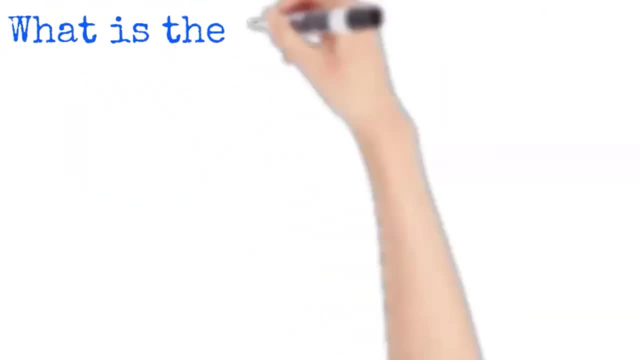 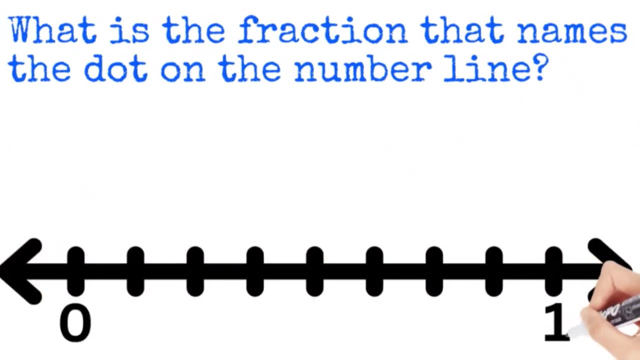 six, Five, six is the fraction that names the dot on the number line. What is the fraction that names the dot on this number line? Okay, remember, from zero to one is my whole and here's your dot. So let's count the pieces that the whole is broken into. So that's four, five, six, seven. 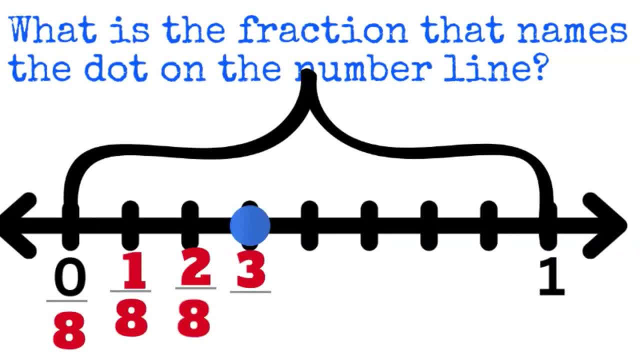 eight equal parts. So eight is my denominator. So that's zero-eighths, one-eighths, two-eighths, and so on, and so on, and so on, until we get to the whole, or eight-eighths, But the dot is actually on. 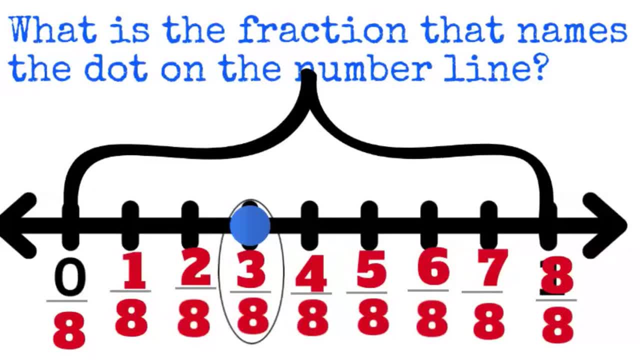 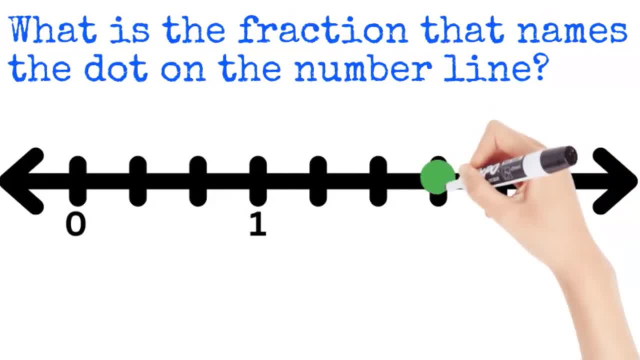 three-eighths. So three-eighths is the fraction that names the dot on the number line. You're doing great. Let's try another one. So the dot this time is way past the whole. Let's see if we can still do this. Yes, we can. So one, two, three, four, five, six, seven, eight, nine, 10,. 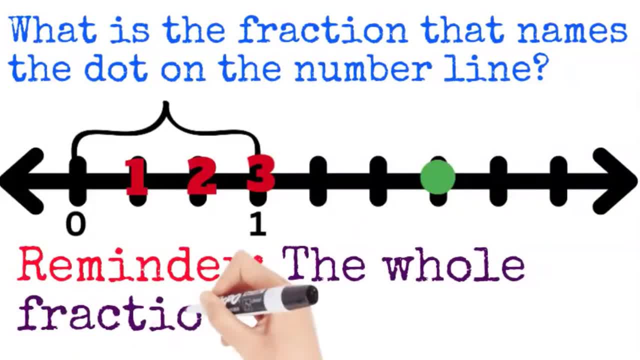 11,, 12,, 13,, 14,, 15,, 16,, 17,, 18,, 19,, 20,, 22,, 23,, 24,, 25,, 26,, 27,, 30,, 32,, 34,, 35,, 37,, 32,, 34,iraoo two. 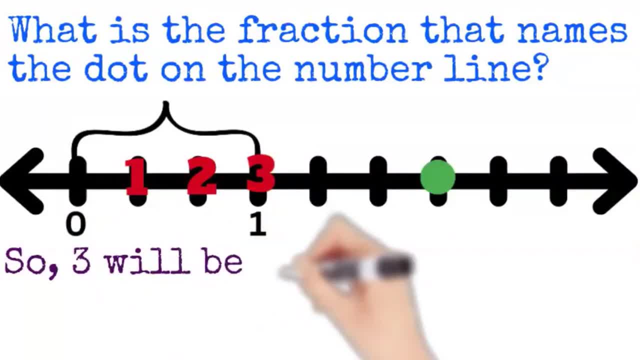 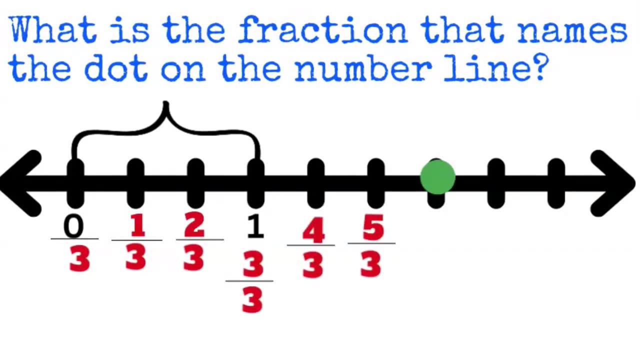 three pieces. Here's your reminder. The whole, the whole fraction, is from zero to one. okay, On this number line the whole is broken into three equal parts. So three will be my denominator, or the number at the bottom of the bar Man of the memorizeDrive. reason to read this question in. for one minute Because I know what book has to be happier than mine. That's funny, But by the end, while developing the equation, it does take a long time understanding the arts and %. just agree tofry read on it easily. Be sure to add the wrong spelling. 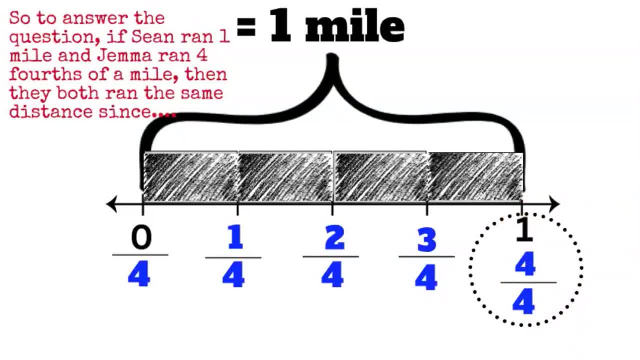 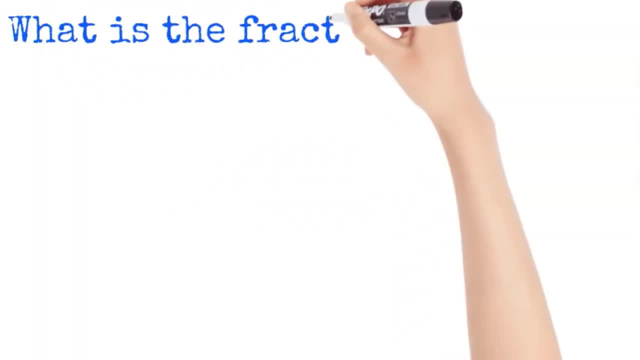 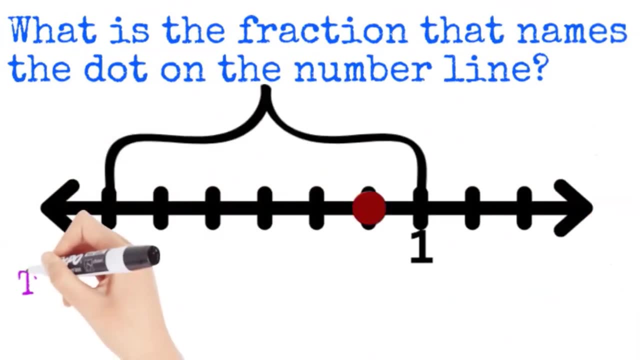 ran the same distance. since one whole is the same as four-fourths, When your numerator denominator are the same, then it's one whole. Let's try this one. What is the fraction that names the dot on the number line? Remember, the number line shows zero to one and the whole is: 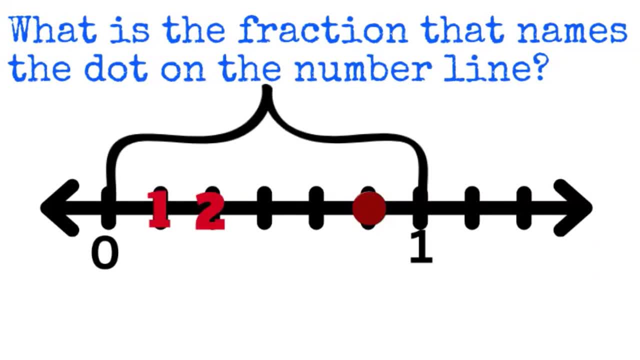 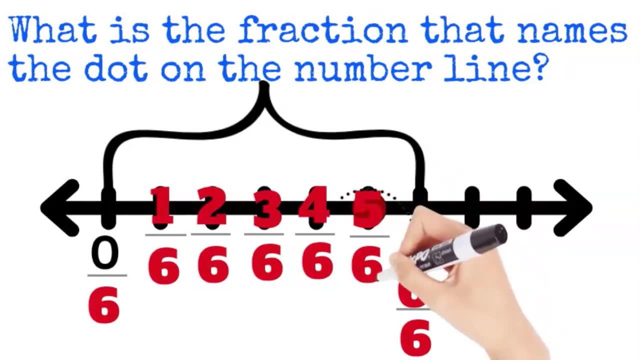 always from zero to one, So we're going to break the whole into pieces to figure out our denominator. In this case there are six equal pieces, So six is my denominator. There's one, six, two, six, three, six, four, six, five, six and six, six would be my whole. However, the dot is on five. 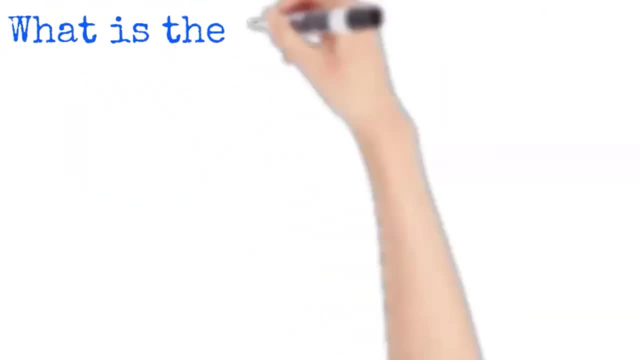 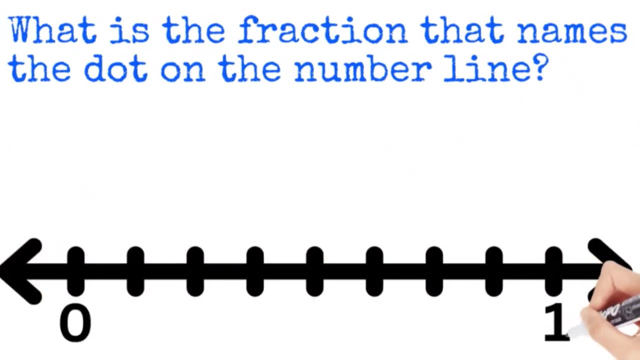 six, Five, six is the fraction that names the dot on the number line. What is the fraction that names the dot on this number line? Okay, remember, from zero to one is my whole and here's your dot. So let's count the pieces that the whole is broken into. So that's four, five, six, seven. 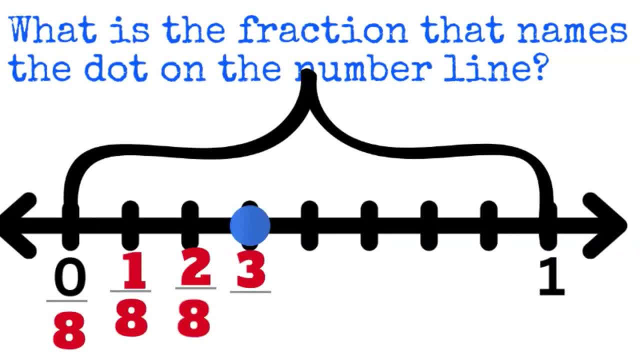 eight equal parts. So eight is my denominator. So that's zero-eighths, one-eighths, two-eighths, and so on, and so on, and so on, until we get to the whole, or eight-eighths, But the dot is actually on. 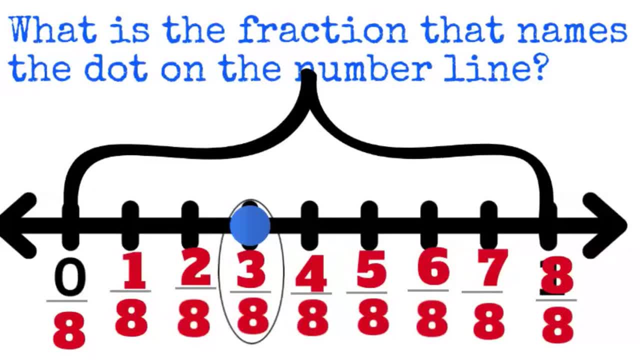 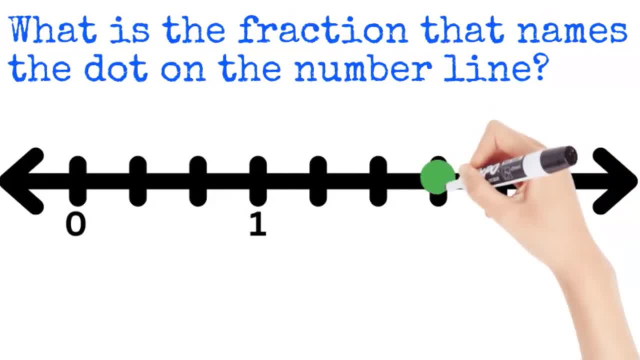 three-eighths. So three-eighths is the fraction that names the dot on the number line. You're doing great. Let's try another one. So the dot this time is way past the whole. Let's see if we can still do this. Yes, we can. So one, two, three, four, five, six, seven, eight, nine, 10,. 12,, 13,, 14,, 15,, 16,, 17,, 18,, 19,, 20,, 21,, 22,, 23,, 24,, 25,, 26,, 27,, 28,, 29,, 30,, 31,, 32,, 3,, 3, pieces. Here's: 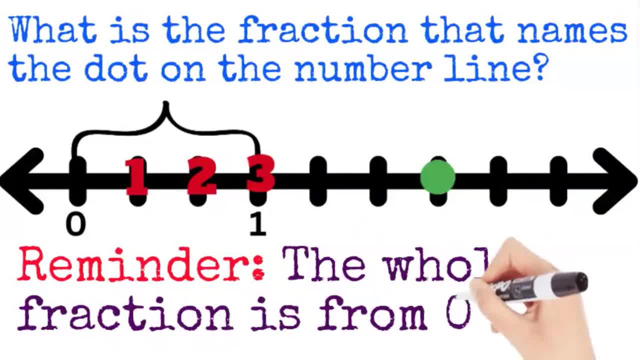 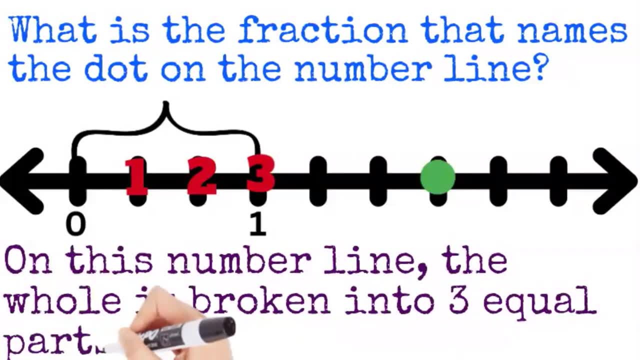 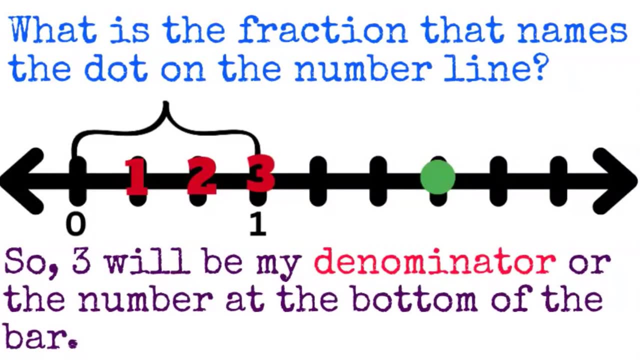 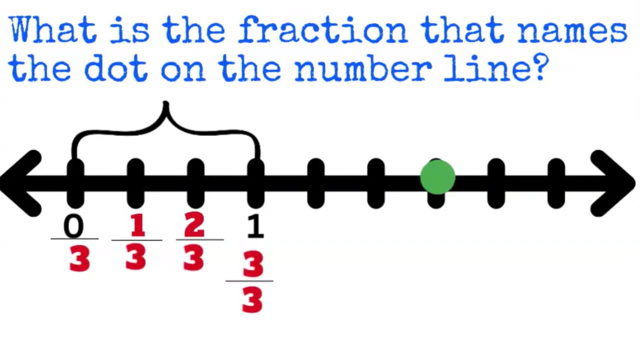 your reminder, The whole, the whole fraction, is from zero to one. Okay, on this number line, the whole is broken into three equal parts. So three will be my denominator, or the number at the bottom of the bar. So that's zero-thirds, one-third, two-thirds and then three-thirds.